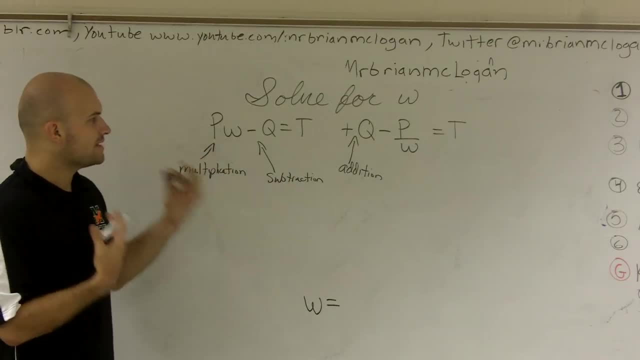 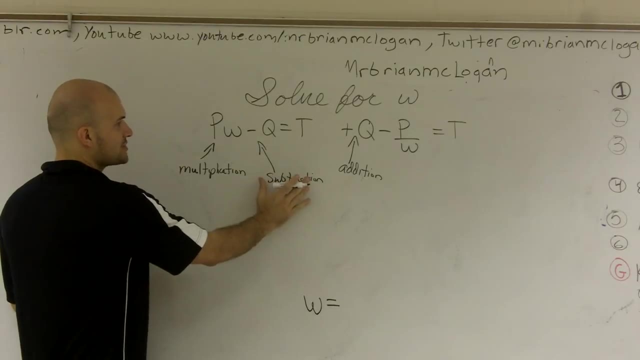 So, first thing, what we want to do is, when we're doing inverse operations- it's kind of like the reverse PEMDAS, reverse order of operations- You always want to undo addition and subtraction first, So I need to undo subtracting by my q. So to do that, I'm going to want to add q. 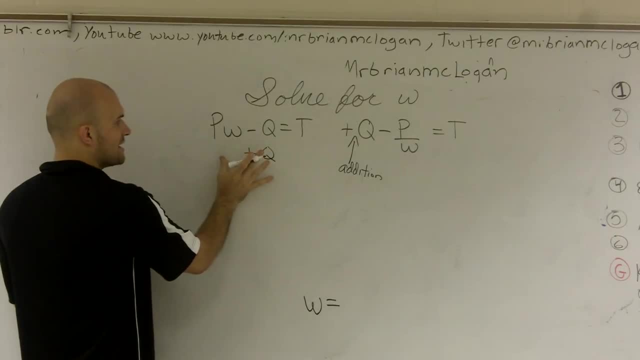 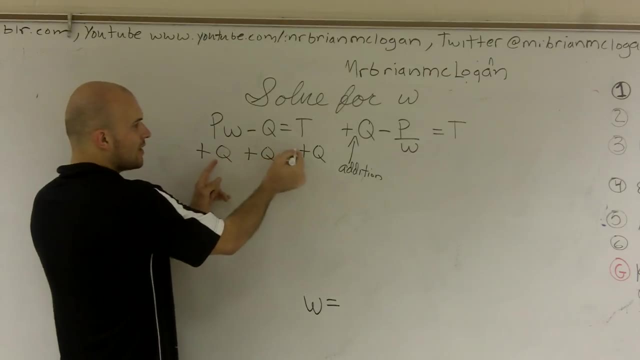 So here I'm going to add q, And remember, whatever you add on the left side, you have to make sure you add to the right side. A lot of students will add a q over here. Well, that's just adding two q's to one side. Now it's uneven. 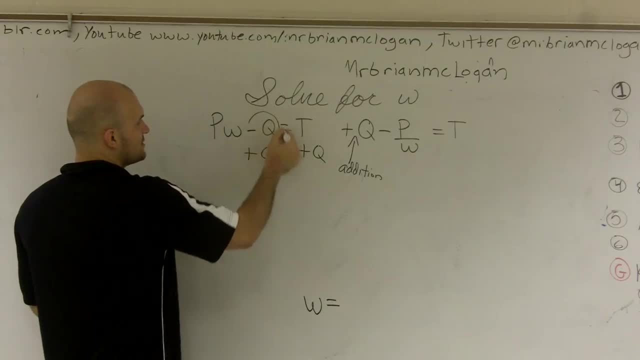 So make sure you only add. See, we want to add these two together, So we want to do this in this case. So now a negative q plus q cancels out to become 0. And that just leaves us with PW equals t plus q, is not w or z or x. 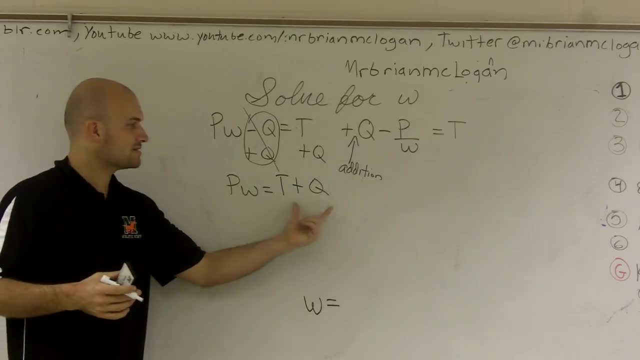 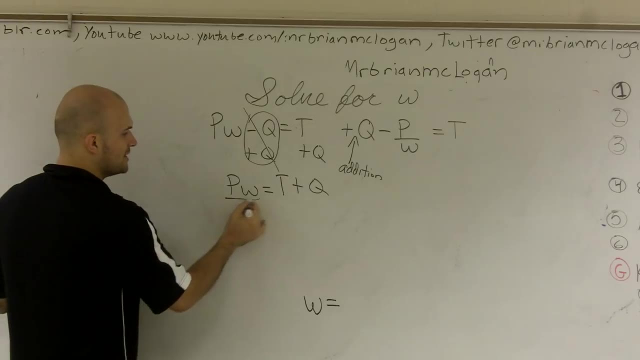 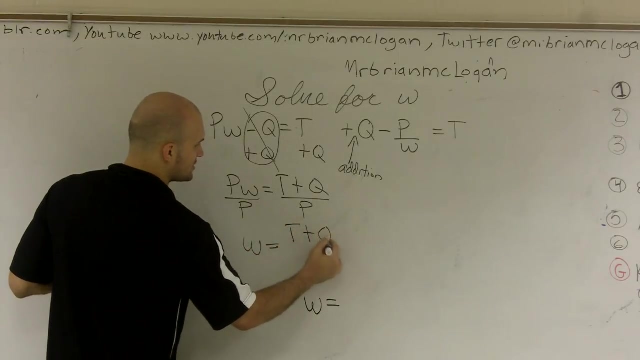 It's just t plus q. We don't know what they represent, so just leave them there. Now, you see, we have multiplication by our p, So to undo multiplication we need to divide by p. So therefore, my final answer is: w equals t plus q, all over p. 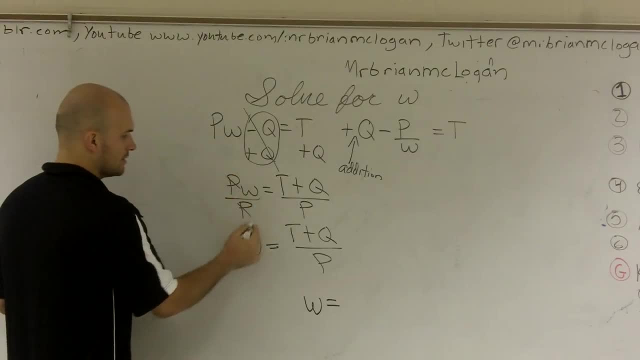 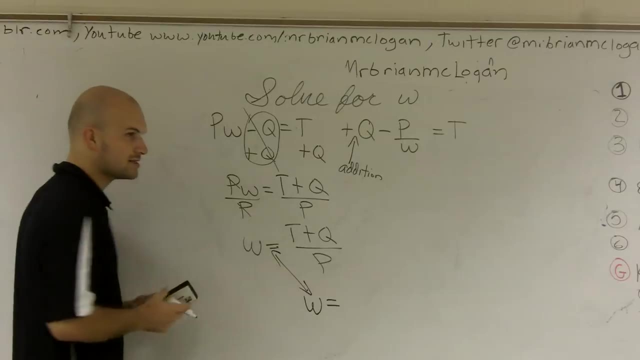 And remember, anything divided by itself is going to equal 1.. So that's why I have that 1 there. But we don't really write 1 times w, We can just write w. And you notice is my answer in: w equals. 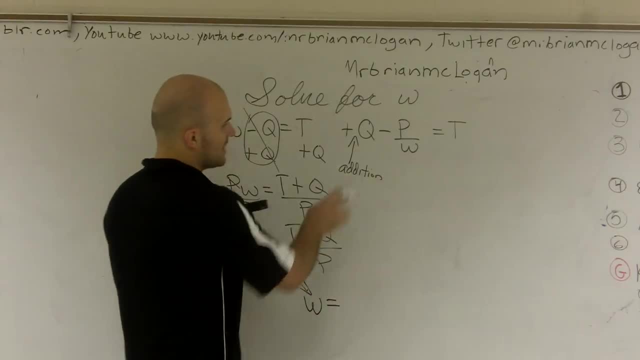 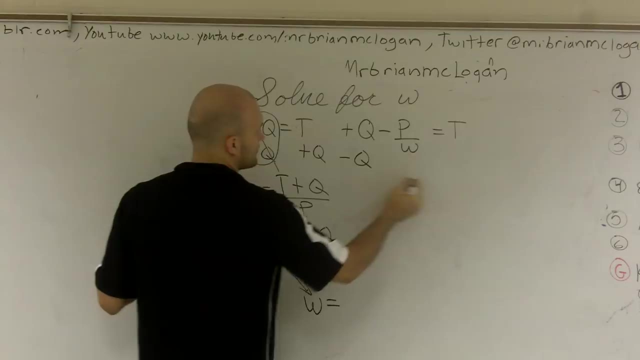 Yes, So we're good, All right. So over here we have this addition. that's starting off right. We want to get rid of addition first, So to do that I'm going to have to subtract by q, So therefore I have a negative p over w. 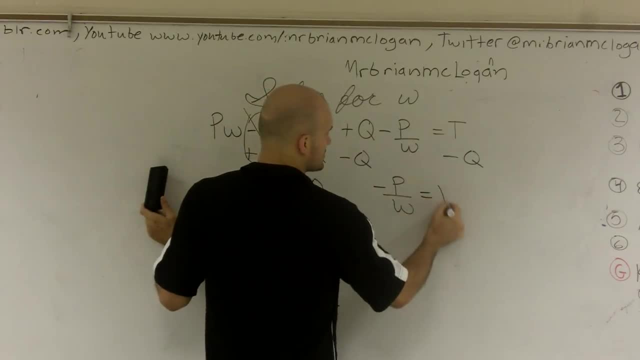 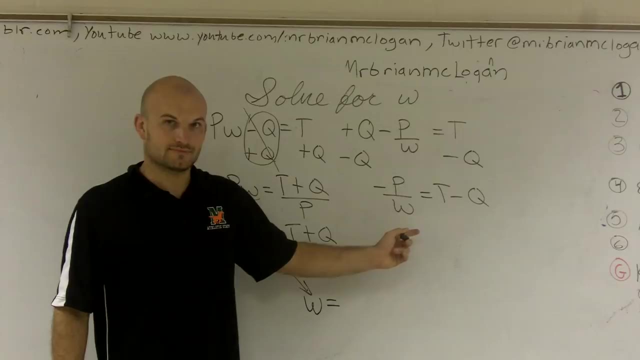 Remember this is a negative, So you've got to keep that negative sign there. It equals t minus q. Now here's where we have a problem. We have this w on the bottom right And we need to get the w off of the bottom right. 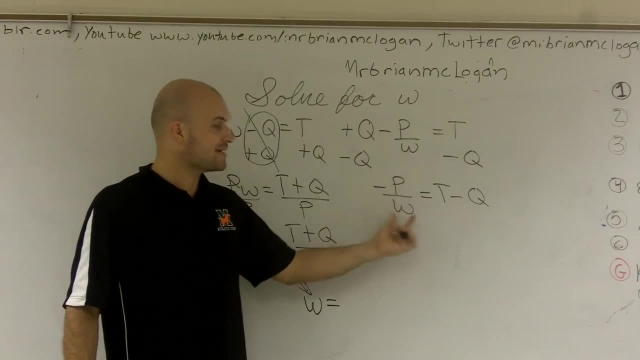 So this is a fraction. What means this is: I'm dividing by w, So I'm going to have to undo this division. So what I'm going to have to do to undo that, I'm going to have to multiply by w on both sides.